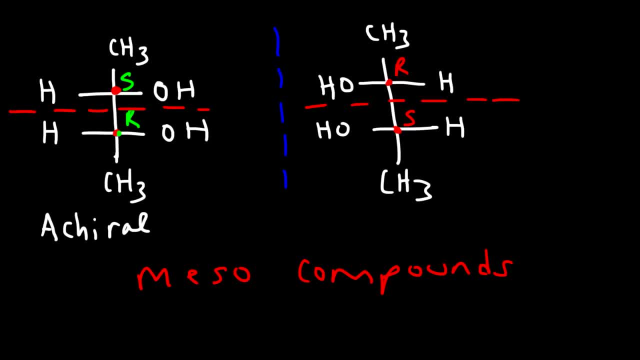 And so mesocompounds are optically inactive, and what this means is that mesocompounds do not have a line of symmetry, So mesocompounds are optically inactive, and what this means is that mesocompounds do not rotate plane polarized light. So make sure you understand that mesocompounds 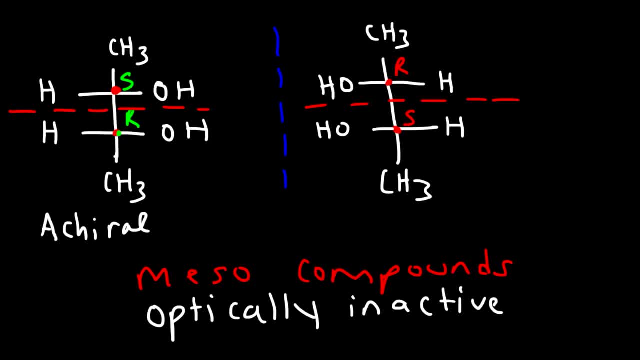 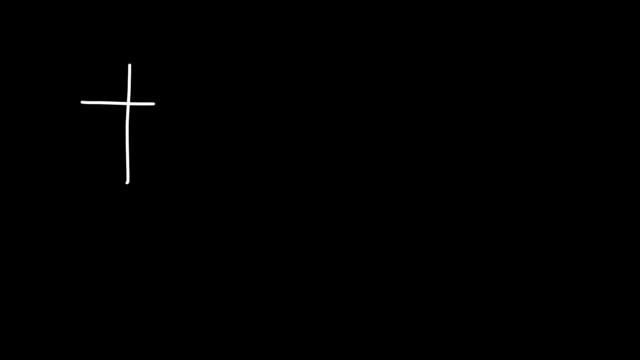 are always optically inactive. And the reason why it has a line of symmetry is you can see that the elements across that internal line of symmetry they're the same. Now let's contrast that with this example. So is this molecule a mesocompound? 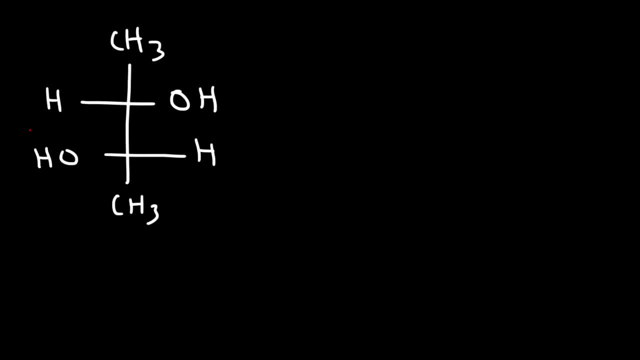 What would you say? So if we draw a line that splits it into two parts, notice that these two are not the same. So there is no internal line of symmetry, which means that the molecule as a whole is chiral and it has two chiral centers. Therefore, we can draw the mirror image of this molecule. 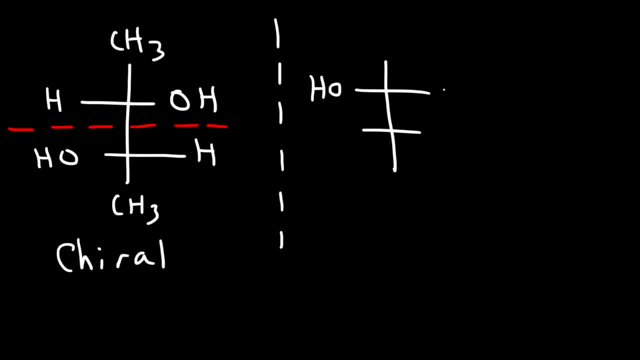 and it's going to be an enantiomer. So enantiomers are chiral molecules and they have chiral centers. Mesocompounds are achiral molecules, but they still have chiral centers. So these two are enantiomers. They don't have an internal line of symmetry. 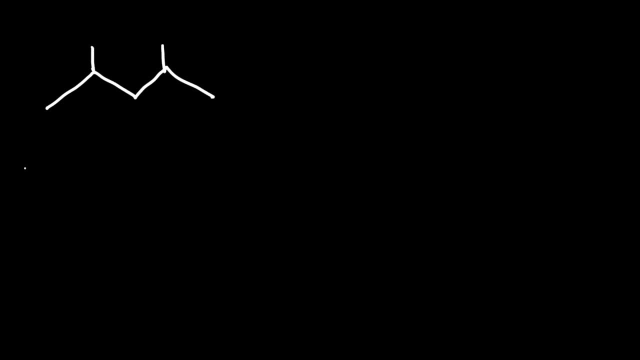 So I'm going to give you a few problems and I want you to determine which of the following molecules are an enantiomer. And I'm going to give you a few problems and I want you to determine which of the following molecules are an enantiomer. 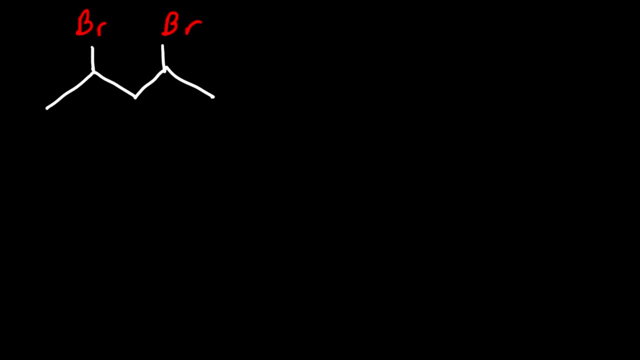 optically active and which ones are optically inactive. So go ahead and try this problem. Feel free to pause the video and work on these examples, And I'm going to give you plenty of examples for you to work on. Okay, Okay. 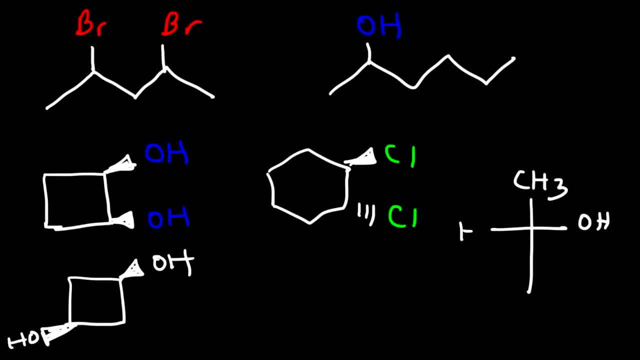 Okay, Okay, Okay, And I think I have one more example, And that should be it. So, looking at the first one, is it optically active or optically inactive? So notice that we do have a line of symmetry. So therefore, this is going to be a mesocompound, which means it's optically inactive. 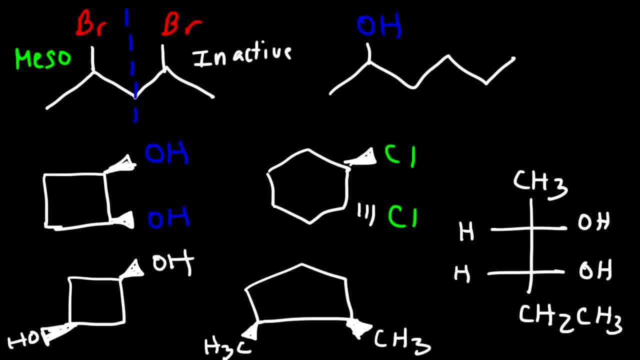 Now what about the structure on the right? There is no line of symmetry, So it's not a mesocompound, which means we can draw the enantiomer if we wanted to. So this is an optically active compound. Now for the next example. notice that we do have a line of symmetry. 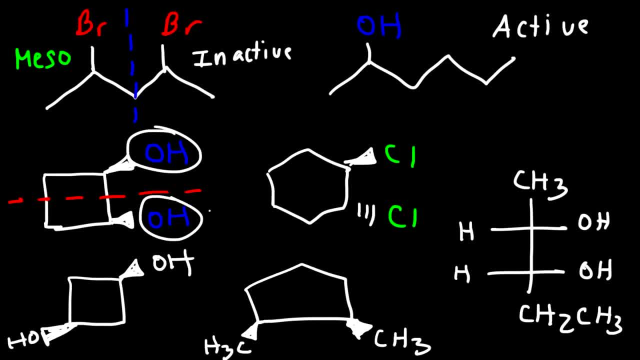 Okay, Okay, Okay. So the OH groups are the same across that internal plane of symmetry, And the same is true for these carbons. So, therefore, this is a mesocompound, And whenever you have a mesocompound, you have an achiral molecule. 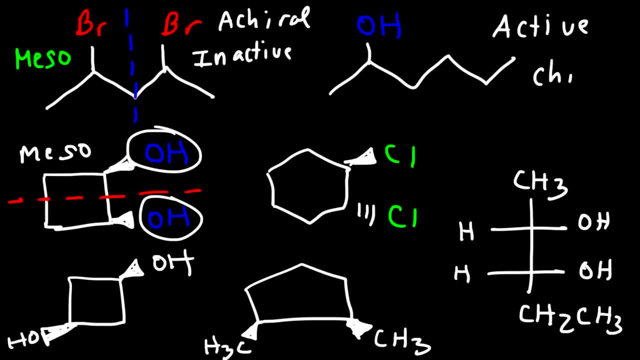 Whereas if you have an optically active molecule, it's a chiral molecule. Now, what about this example? Notice that we do not have, rather, an internal plane of symmetry, Because here the chlorine is in the front, now here it's in the back or going into the 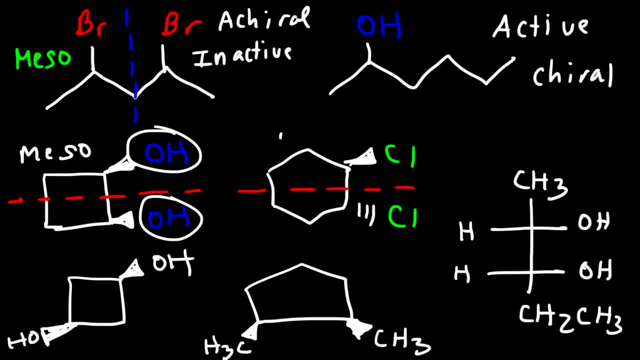 page. So therefore, this is not meso, which means it's optically active. Now, for this example, we do have an internal line of symmetry, And so this is a mesocompound, which means it's optically inactive. 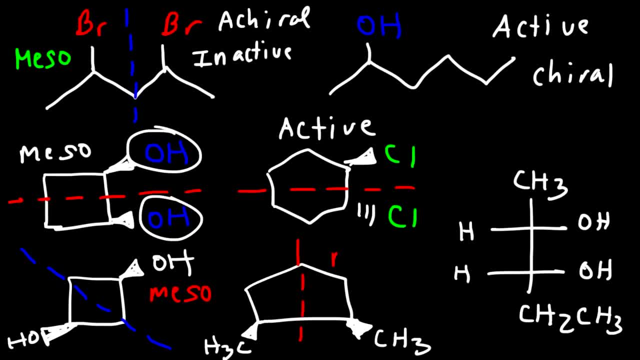 And here is another mesocompound: There's an internal line of symmetry. Now, what about this one? Is this a mesocompound? It turns out that it's not, Even though the H is the same across the line and the OH is the same too. the methyl group.